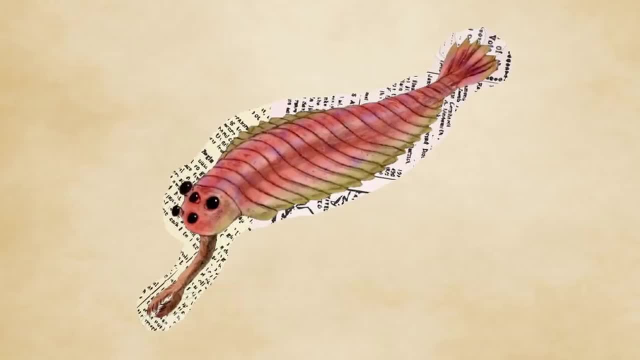 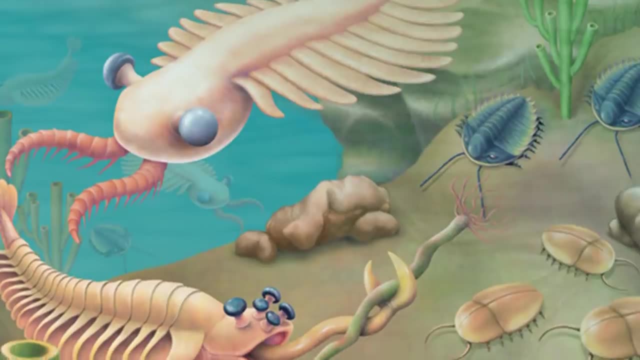 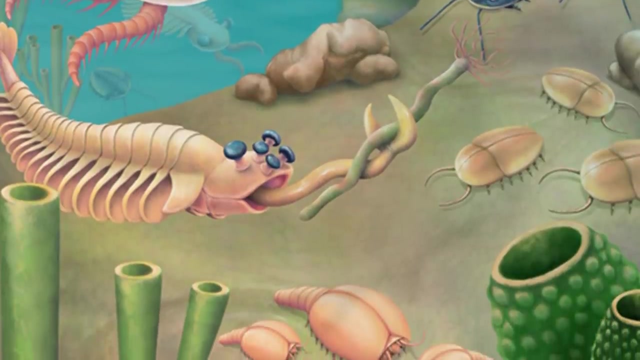 or even fan favorite Hallucigenia are still here. But even here, more than 500 million years ago, is not where animal life starts. Yes, it may have been an explosion, but you still need a fuse to set off a bomb. There was a source before this. it's time to travel. 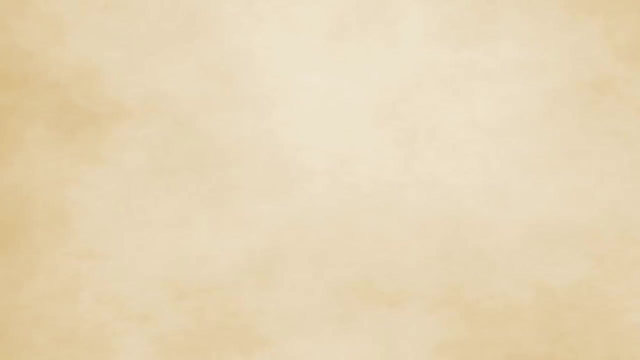 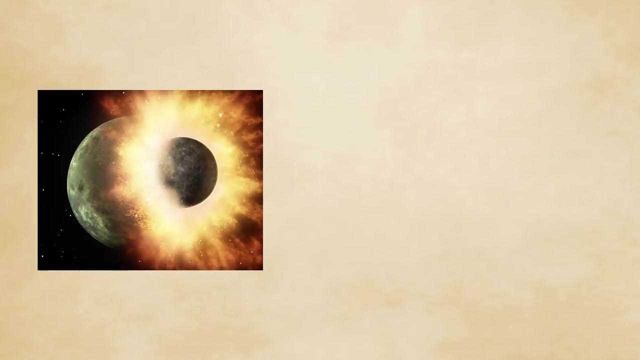 even further back to Pre-Cambrian time Just to get a little glimpse at the scale we are at now. the Pre-Cambrian lasted in between the creation of Earth to the Cambrian Eclipse and the Earth's exodus. So from the Earth to the Earth, there's only one way to get there. 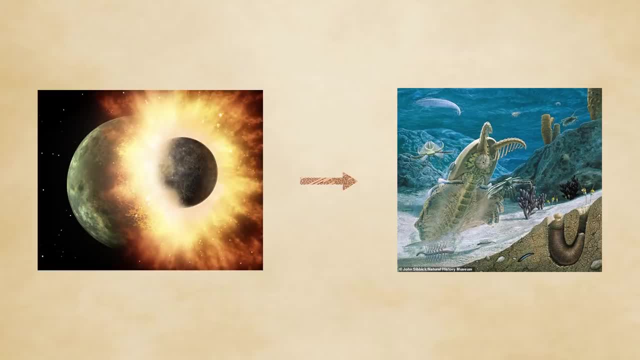 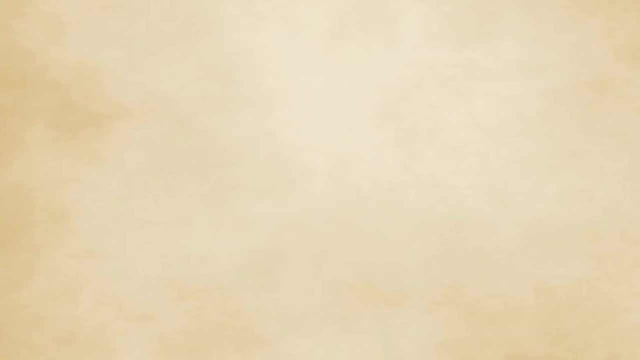 the Cambrian Explosion, which is a time span of about, you know, 4 billion years. The scale of geologic time is so large. at this point we have to unpack some new units of measurement. It's not really adequate to use geological periods or even geological eras. We've now moved on to eons. You 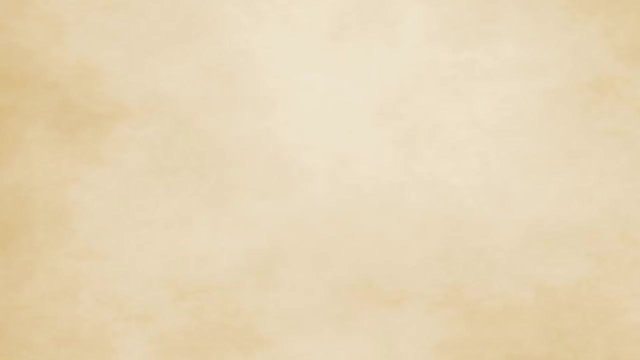 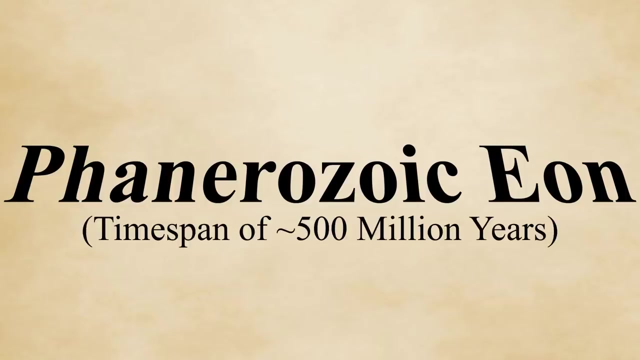 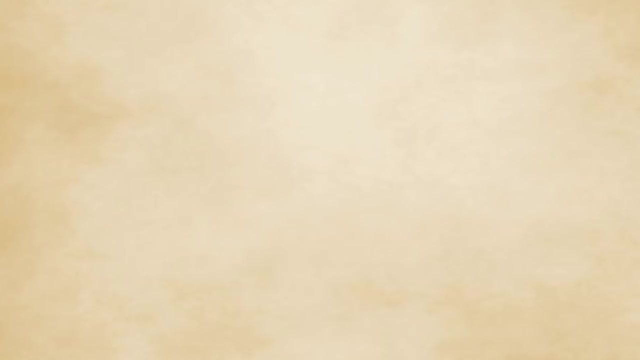 heard right eons. Once more to give some perspective. the most current eon that you and I live in is the Phanerozoic, which started with the Cambrian 541 million years ago. The three earlier eons were all in the Precambrian, each one in descending order having a more sinister name. 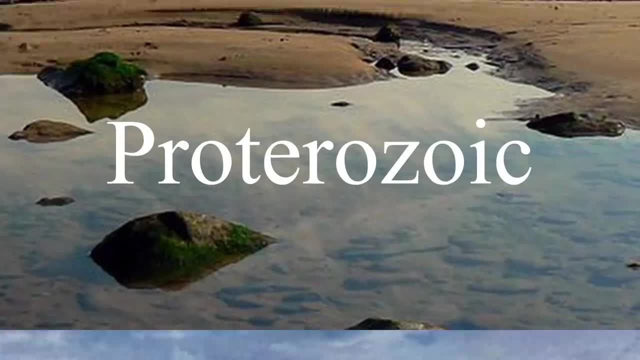 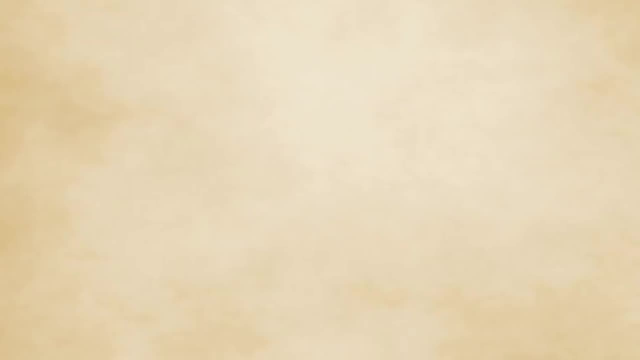 with the Proterozoic being the closest to us, followed by the Archean and finally the Hadean, which, according to the internet, looked like this: Now, the first actual signs of life started in the Archean eon 3.7 billion years ago. 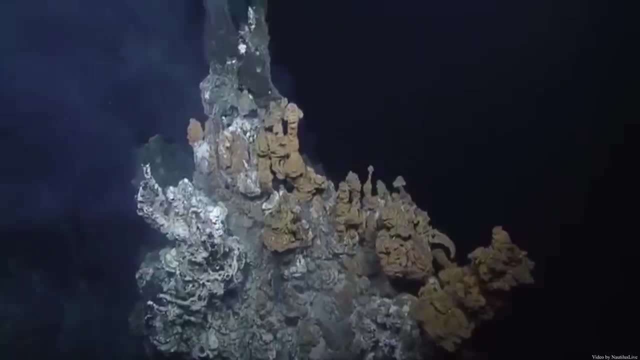 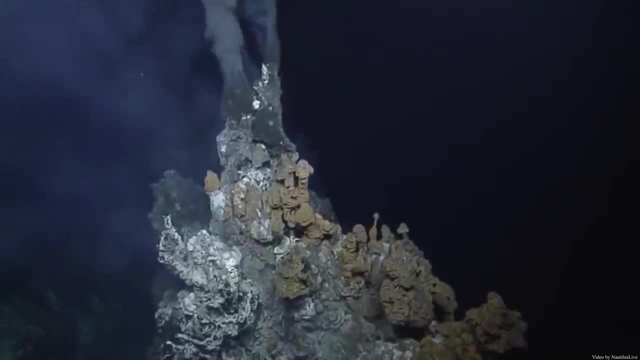 The actual lifeforms can only be theorized and their origins are another video for themselves, but it's probable they were bacteria who got nourishment from the hydrothermal vents of the ocean abyss, But from primordial stones. in Greenland we can find the first recorded organisms. 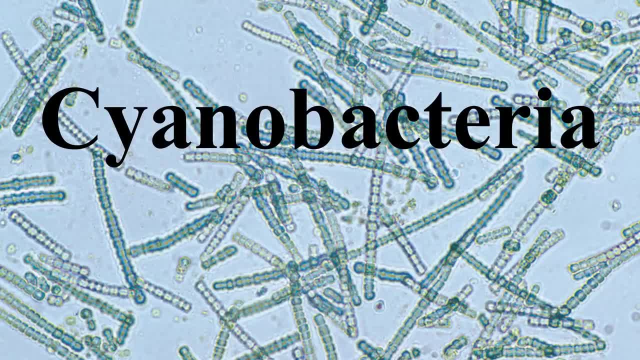 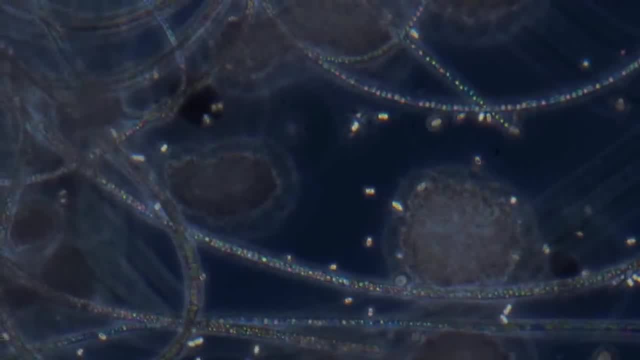 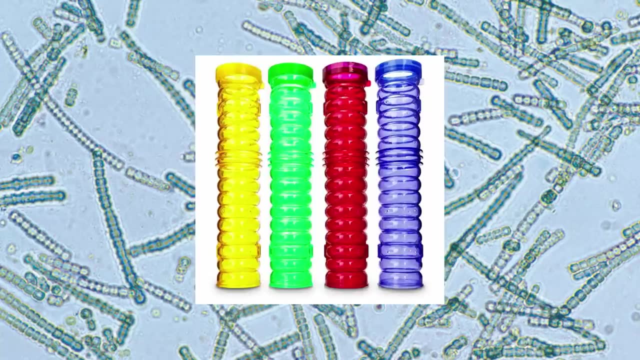 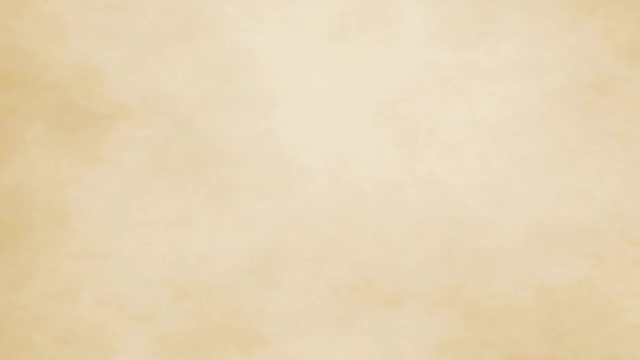 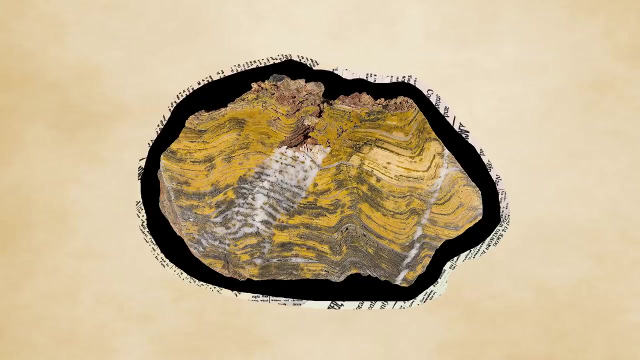 Prepare yourselves for cyanobacteria, aka blue-green algae. Not exactly the most impressive of entities, I know, but they still took the first steps. Cyanobacteria also leave behind interesting traces of their existence, being scrematolites. These scrematolites are the work of bacteria slowly building up layers. 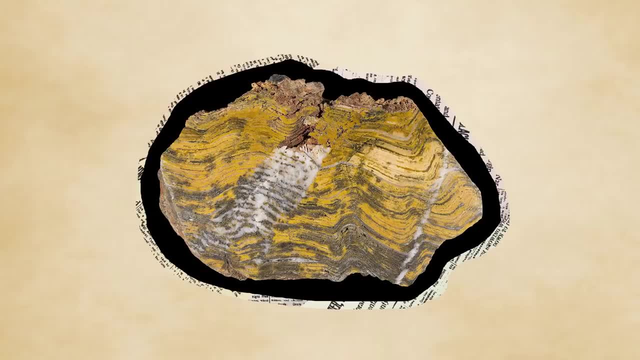 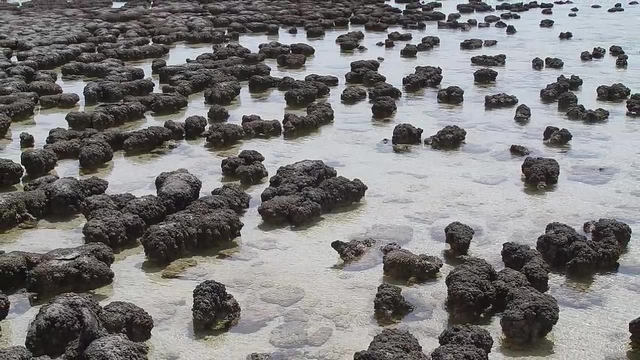 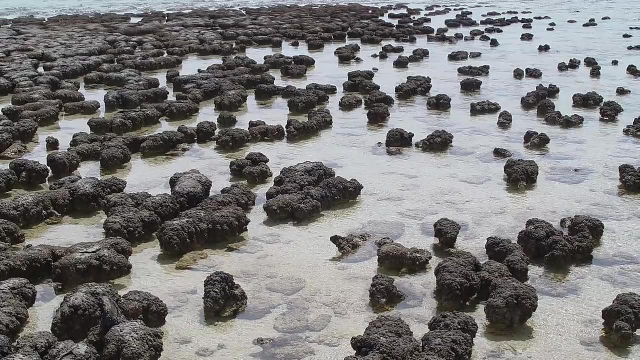 and layers of minerals that get stuck together by the bacteria's adhesive compounds forming these structures. Scrematolites, still exist today, slowly being formed in places like Shark Bay, Australia. Just remember: life like this has existed, unchanging, for billions of years Now. as much as I love praising cyanobacteria, they aren't exactly the first. 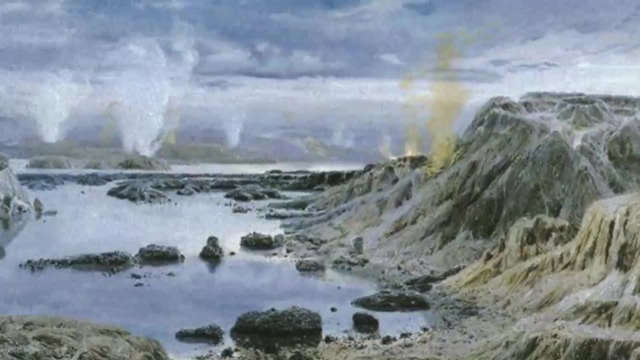 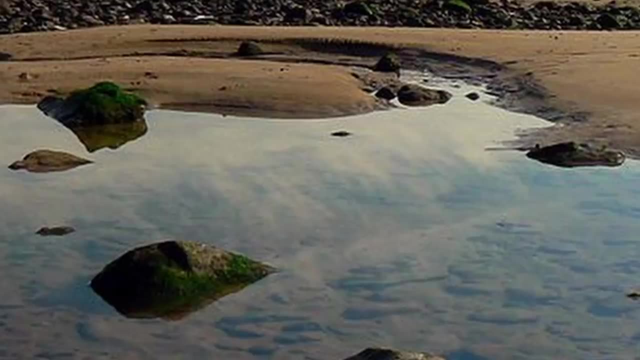 animals, because they aren't animals, they're bacteria. So I know I'm asking a lot, but let's zoom forward a few billion years later. Now we're in the early Proterozoic Eon. Before this time the Earth's ozone layer was so thin and oxygenless, only tough little. 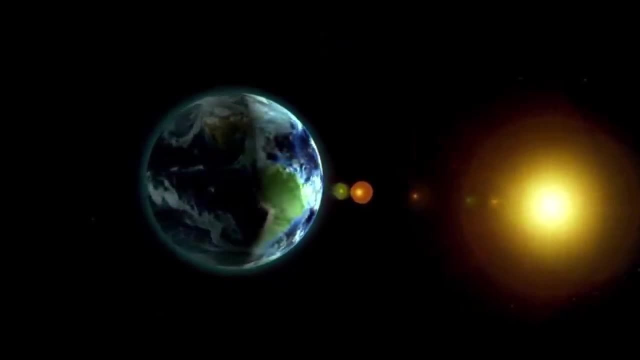 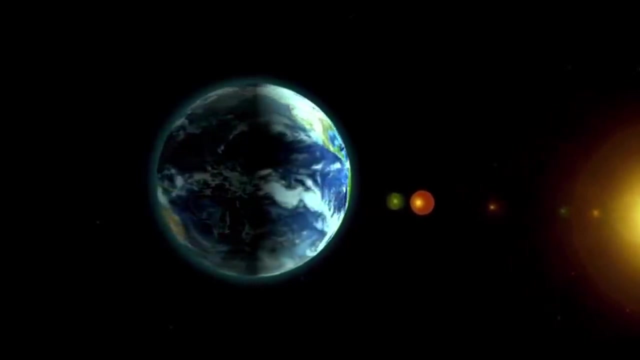 prokaryotes could exist, But eventually, thanks to our heroes cyanobacteria, who produce oxygen and dump it into our atmosphere, the first eukaryotes with cells similar to ours spawned in this new oxygenated world. The world was also really, really cold. 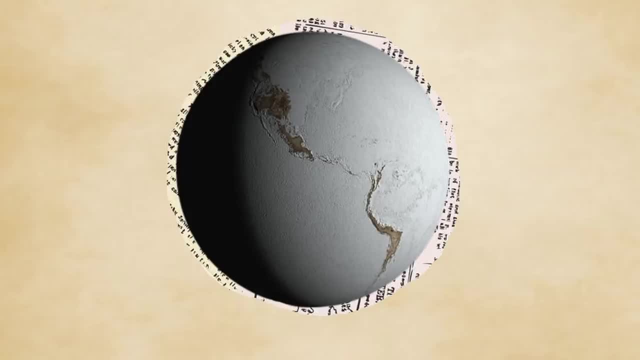 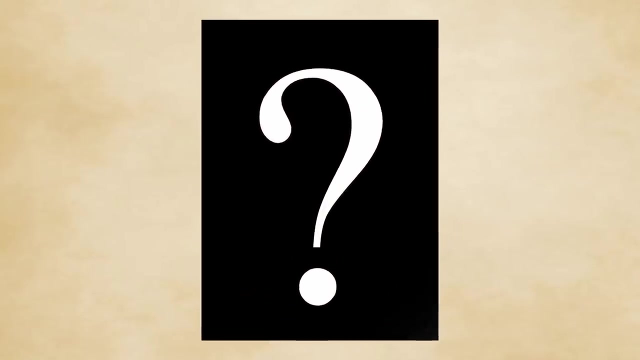 Climate mishap had formed what would be known as Snowball Earth, where the whole globe was essentially permanently covered in an icy winter. Yet it is in these icy waters where the first animals would spawn, Gaze upon zoological genesis with the sponge Indeed before mammals. 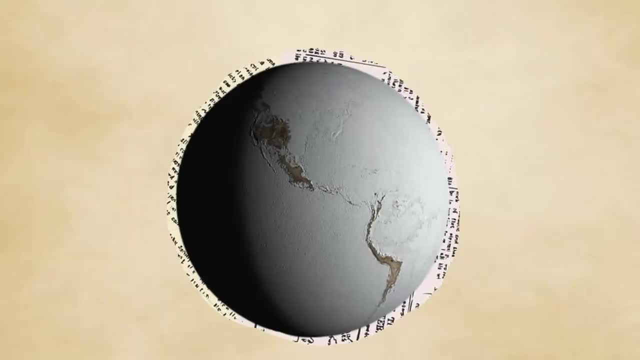 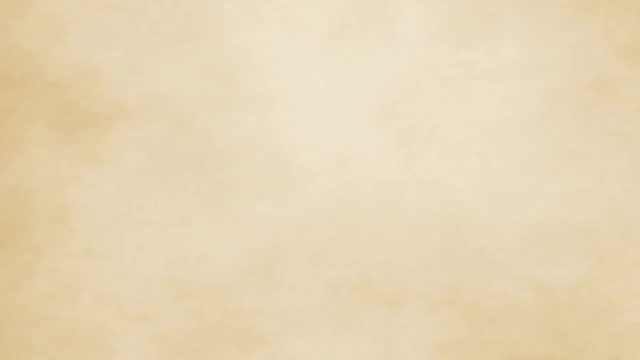 or even reptiles. there was SpongeBob on a giant frozen snowball hurtling through space. Now, as much as sponges are amazing, they aren't. So let's move further on. where the world gets a bit warmer in the Ediacaran Period. It is here where the 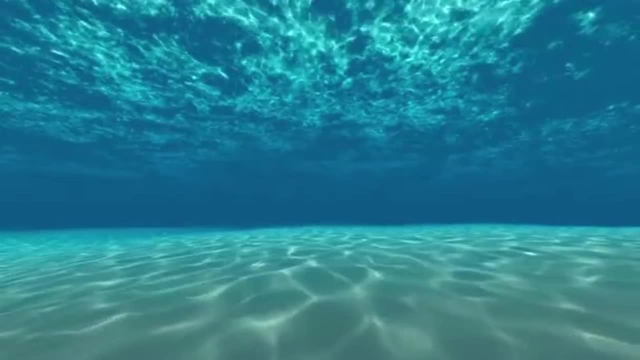 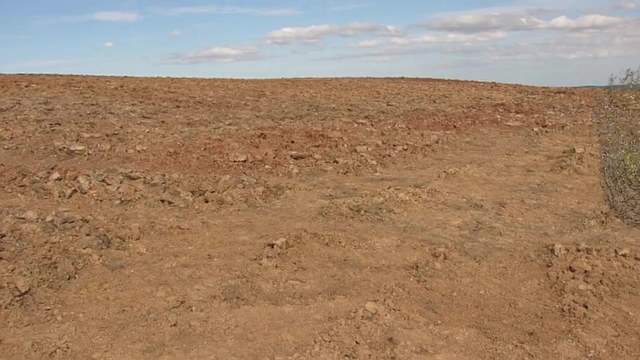 first, animals will evolve into a select few forms in the Precambrian Ocean. I say ocean only, of course, because even though the seas might be tolerable, the land was still barren of any complex life, even of the comical tumbleweed. 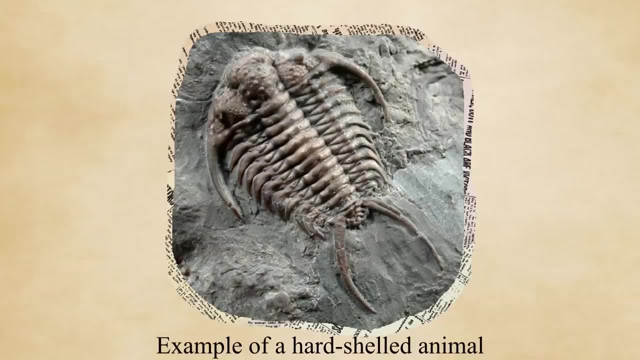 Another quick tip is most of these creatures are boneless. The collagen that would allow Cambrian life to have hard bodies and flourish into many different shapes was not there, leaving many very simplistic and not very mobile. Actually, most of them don't move Like at all. 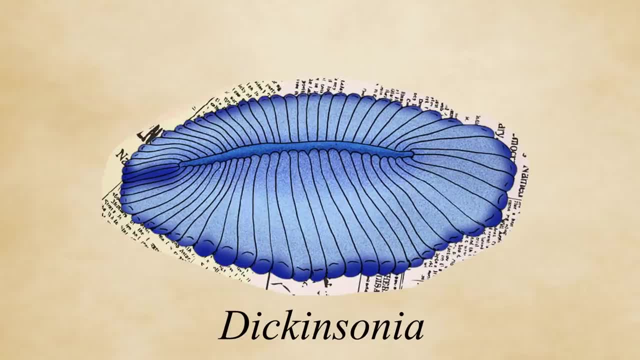 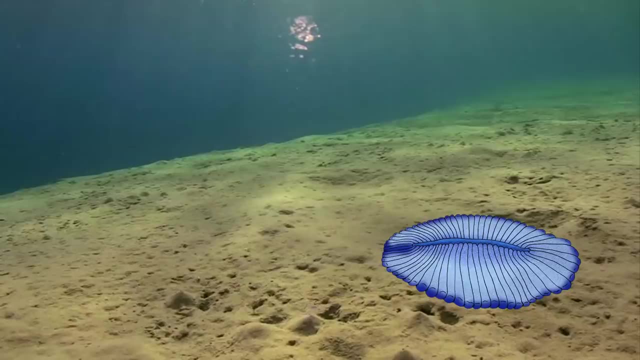 Take, for example, Dickinsonia. This up to 4 foot wide oval had been incessantly debated on whether it was an animal or not, but a fossil showed this creature had cholesterol in its body, something only found in animals. Of course, it just barely counts as one. It's so primitive that it isn't even completely. 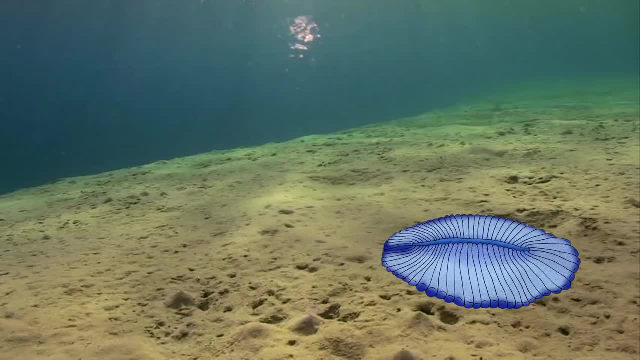 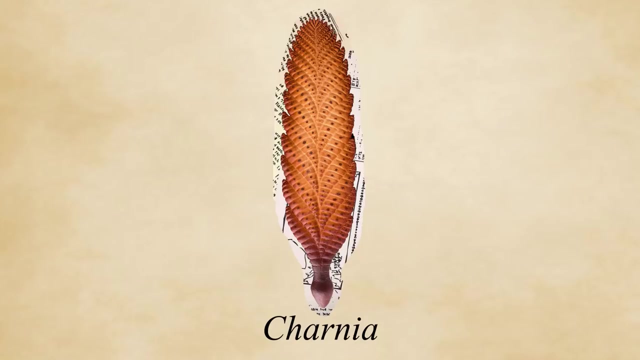 symmetrical, and you probably would mistake it for some sort of sea pancake, since all it does is just sit there Once more. behold your ancestors. Some early creatures were so imaginary- they were basically just plants. Carnia was actually the first pre-Cambrian fossil. 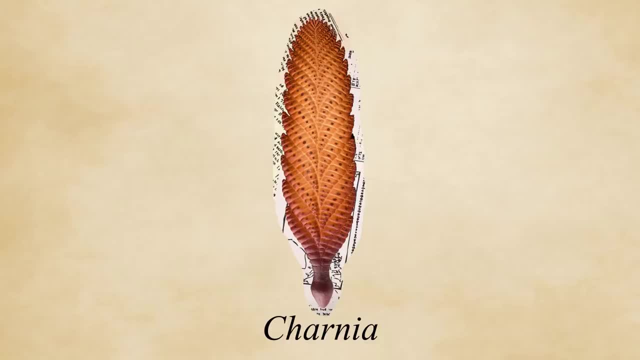 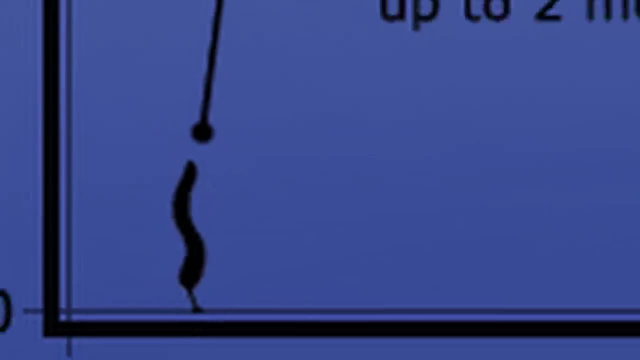 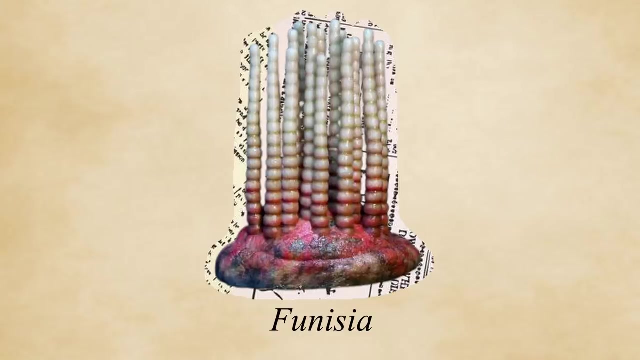 discovered and looks and acts more like a fern than an animal. These plant-like creatures could also range in size greatly. The first specimen was just a few centimeters long, while other specimens could stand taller than a man. Phoenicia also looks like some alien plant, but it is in fact many worm-like creatures grouped together. 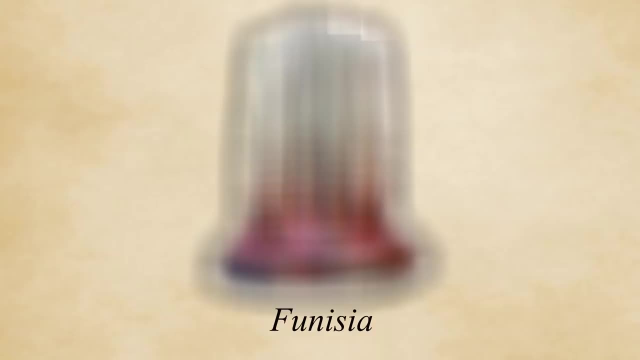 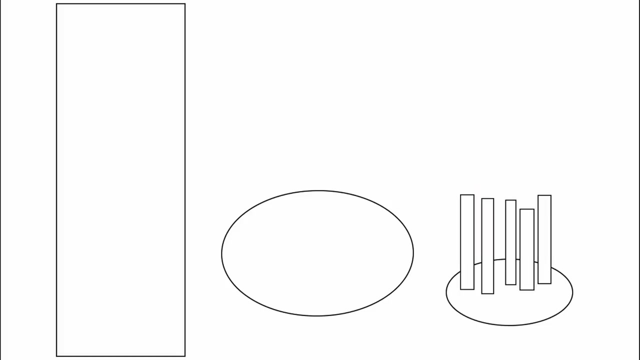 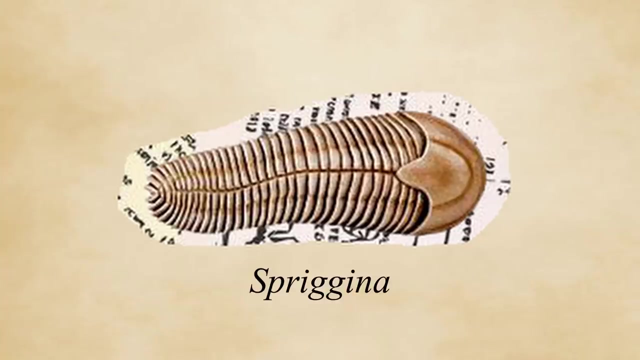 You might actually have to blur this little picture because, although it doesn't look like it, Phoenicia might have been the first animals to sexually reproduce. Compared to these static basic shapes, this creature called a Spurigina doesn't grow any longer than 5 centimeters, but they are some revolutionary animals. 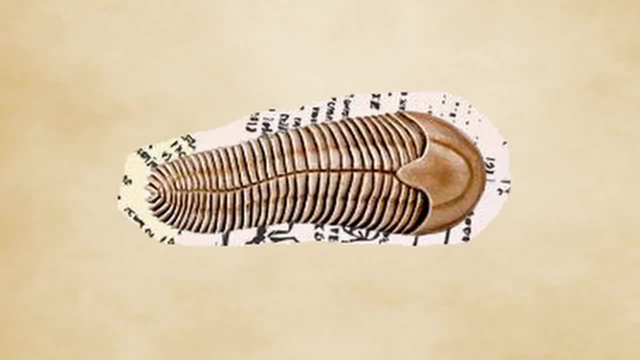 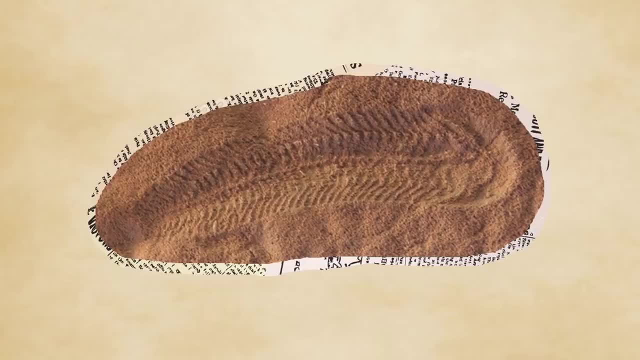 They have a worm-like segmented body and what appears to be one of the first heads on earth. This general body plan of a bilaterally symmetrical form with a head on one end will repeat for the next 600 million years on a vast majority of animals. 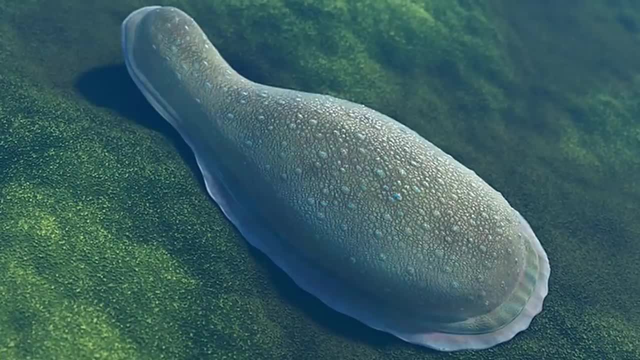 Another precedent setter was the Chimborella. These animals might have acted as some of the world's first bottom feeders, crawling along shallow seafloors and grazing on colonies of microbes. And, of course, some creatures from the pre-Cambrian in fact still remain. You guessed? 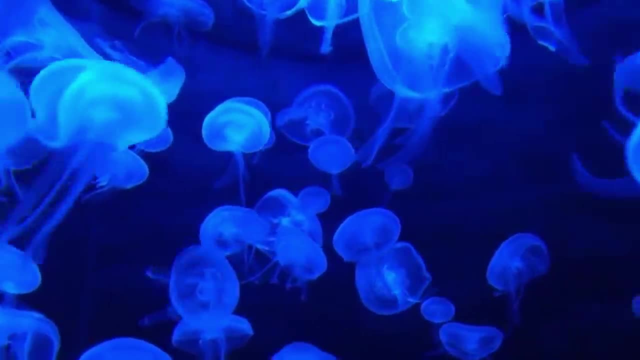 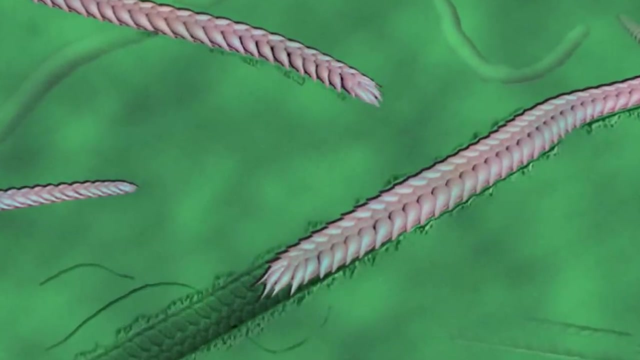 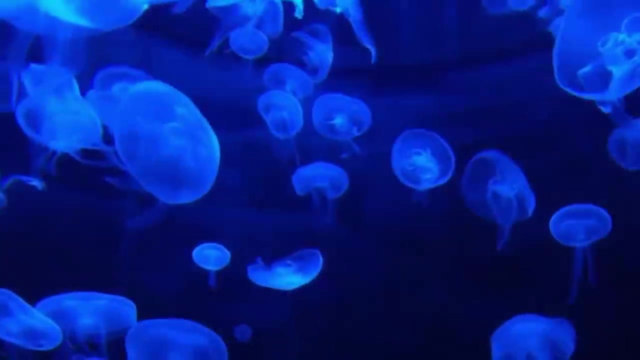 it. the seemingly eternal jellyfish has been floating around doing nothing for a while. Trace fossils of narrow line-like markings in the seabed reveal. even back then there were still worms not dissimilar to some deep sea worms of today, who burrow through ocean dirt Along with